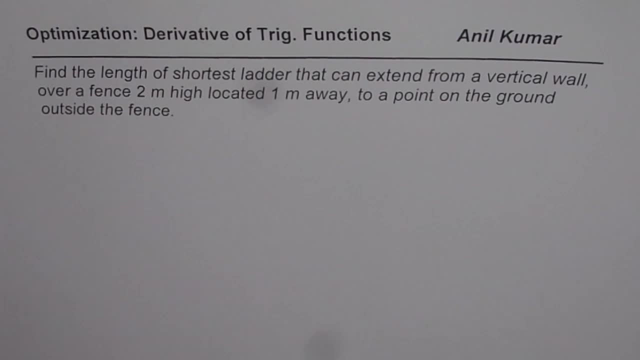 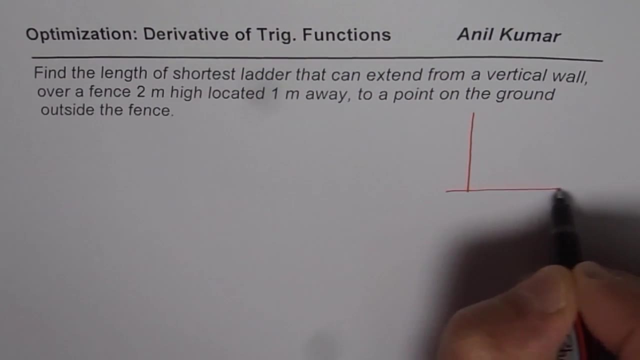 away to a point on the ground outside the fence. So let me make a diagram to represent the situation so it's absolutely clear to you. So think like this, that we have a ladder which is like this And what we have here is a fence in between, And the fence is about two meter high, And that is the fence which. 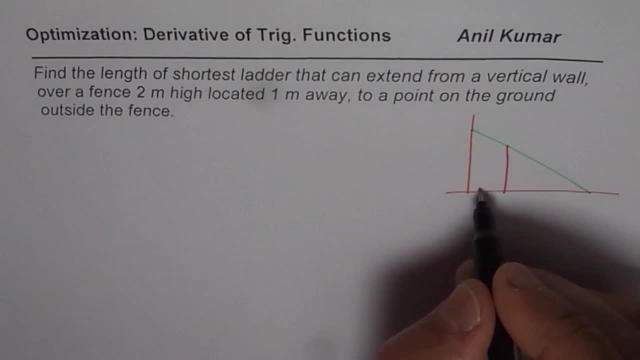 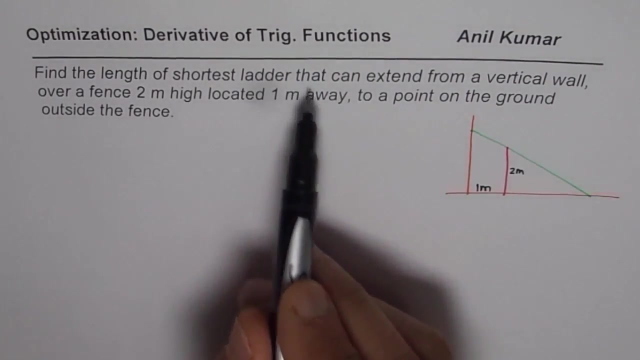 is two meter high and it is one meter away from the wall. So it's one meter away and it is two meter high. So that is the fence and this is the ladder which we have. So let's read the question: Find the length of the shortest ladder that can extend from. 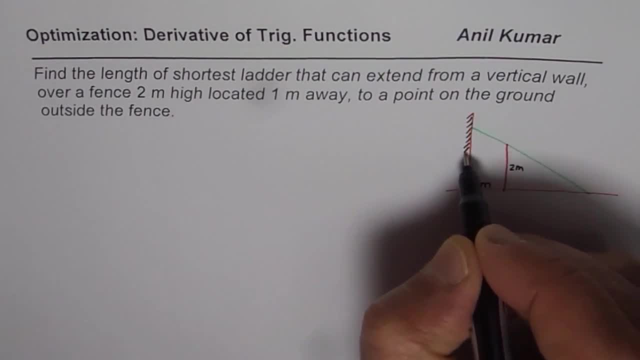 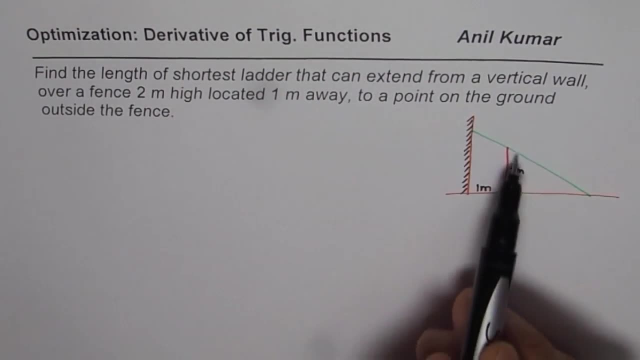 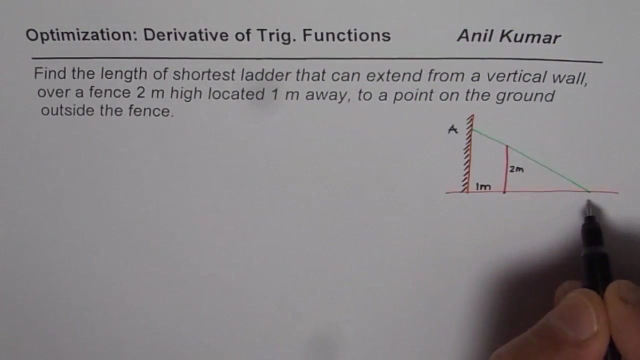 a vertical wall. so that is the vertical wall we're talking about over a fence, two meter high, located one meter away. So this fence is one meter away from the wall And that ladder is to be extended from a vertical wall. So that is how the ladder is. So let us say the points A and B represents the length of 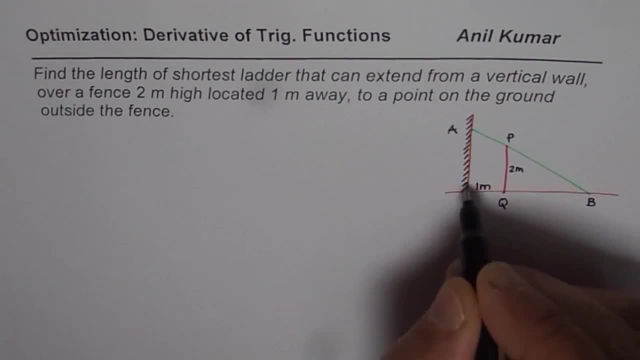 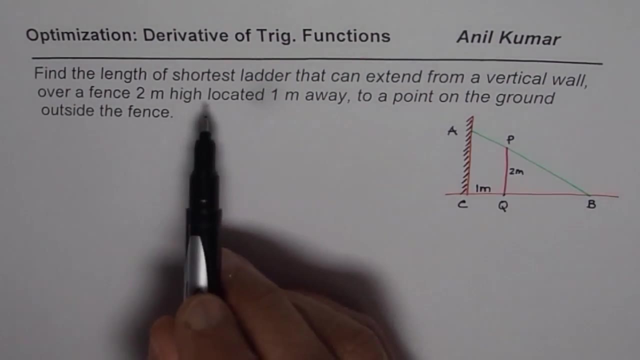 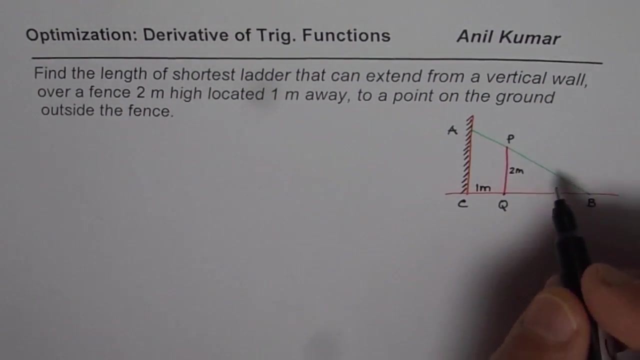 the ladder. Let's call this point as PQ and I'll just name this as C here, So that diagram clearly indicates or represents the situation. Now the question before us is: we need to find the shortest length of this ladder. Now we'll have let this angle 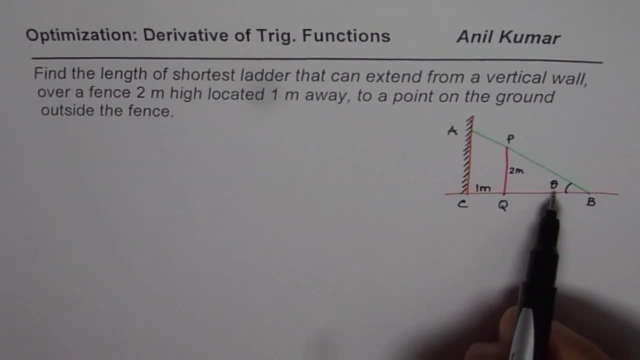 be theta, so we can write a relation in terms of theta for length of the ladder. Now some of you can actually pause the video, try it out and then look into my suggestions. Now, in this particular case, we can write length of the ladder in terms of angle- theta, Let. me show you how. 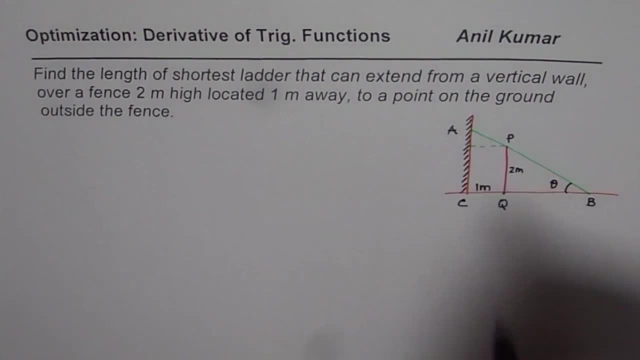 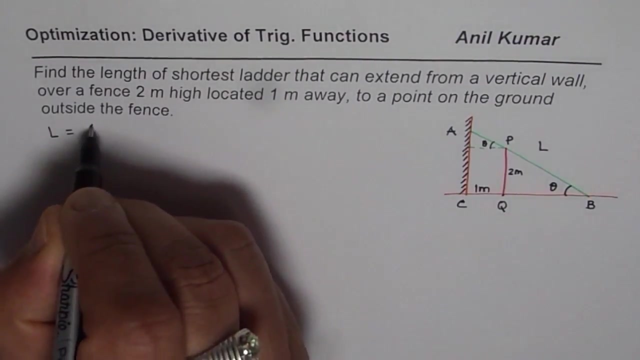 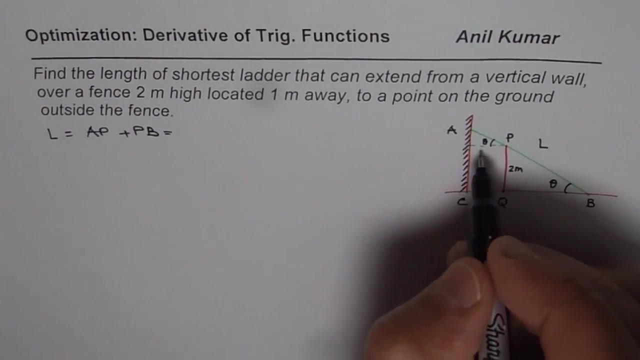 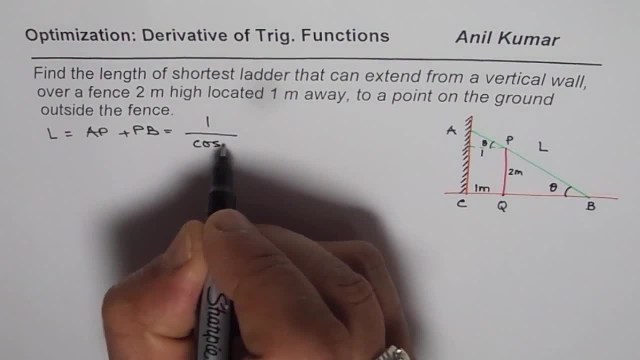 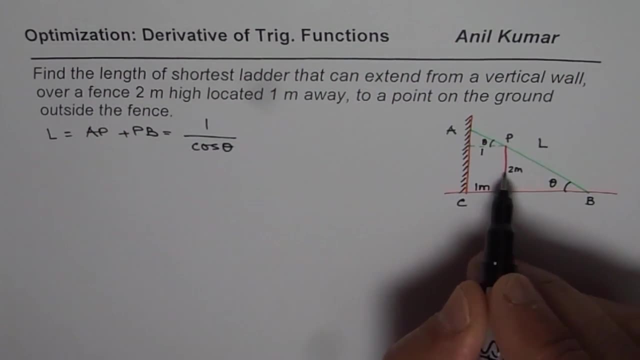 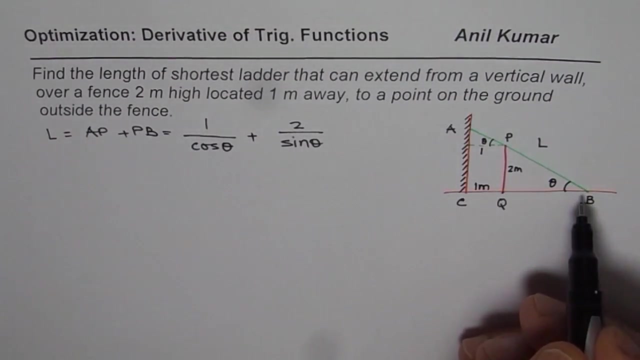 theta. So I could write this as 1 divided by cos of theta And Pb opposite side to theta is 2 meters sine theta is now in question, So it will be Pb will be 2 divided by sine of theta. So that is how you can find length of the ladder as related with the angle theta. 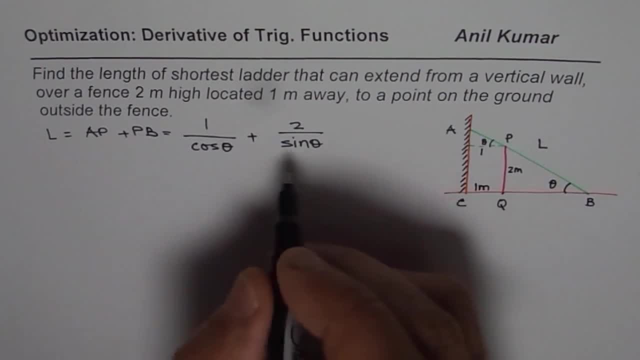 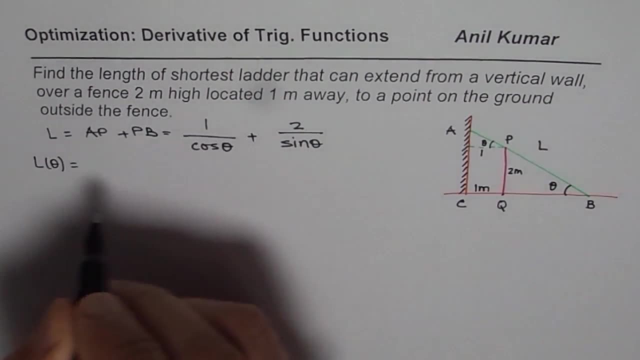 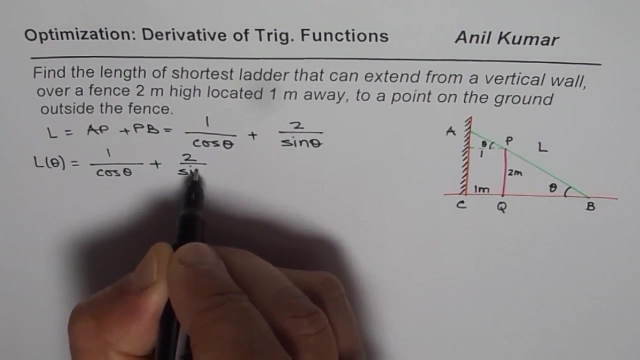 itself. Now it is very important to understand that this expression which we have in terms of theta- so length in terms of theta- is a function where this is equal to 1 over cos theta plus 2 over sine theta. Now here, angle theta is between 0 to 90 degrees right It. 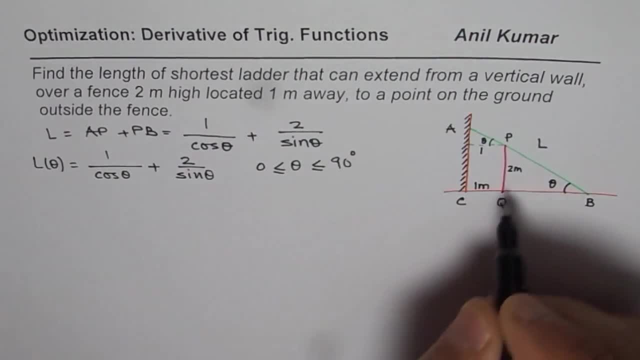 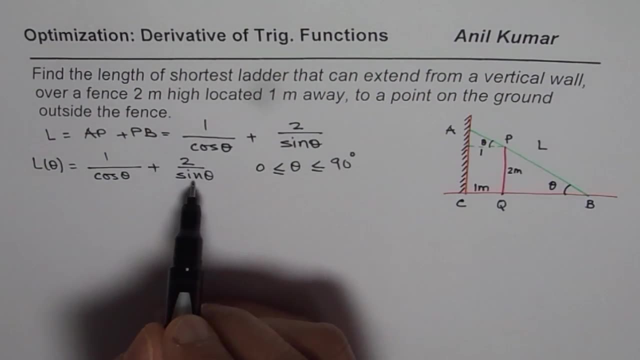 is between 0 to 90 degrees. If I substitute 0 here, then I get the length of the ladder. then what happens? For 0, sine is 0,, so we get infinite length. And for 90, cos is 0,. 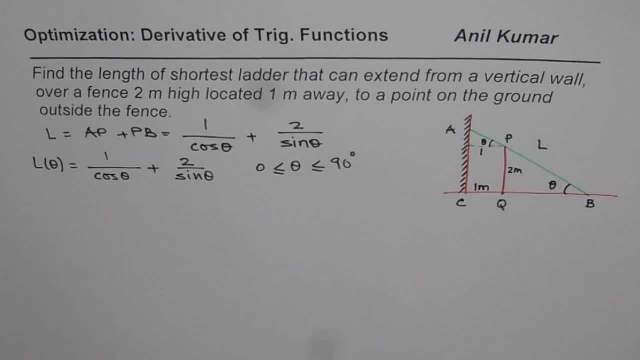 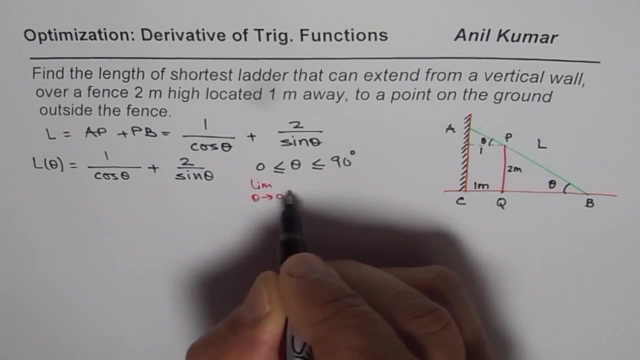 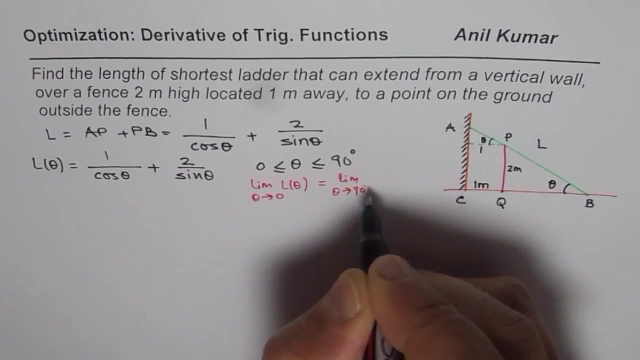 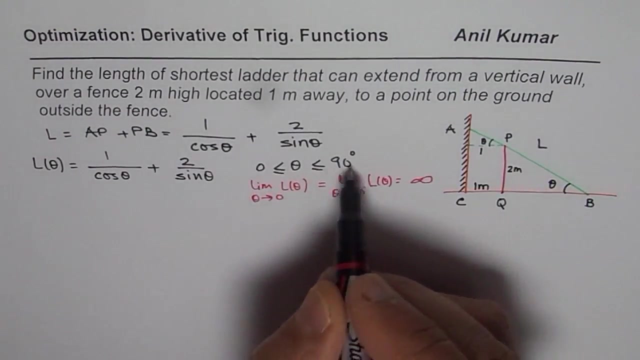 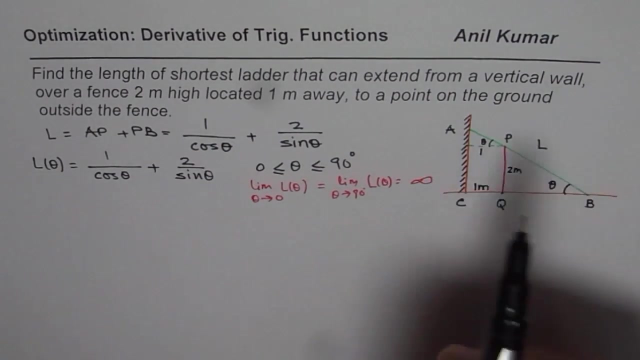 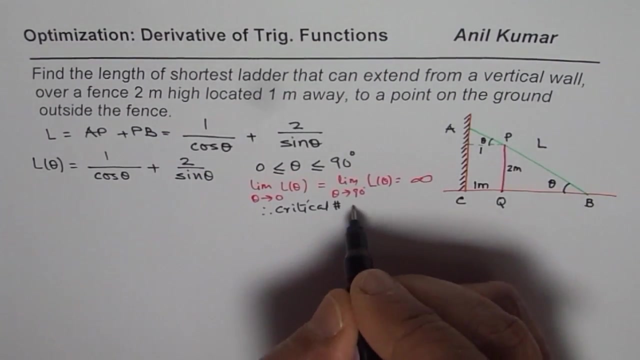 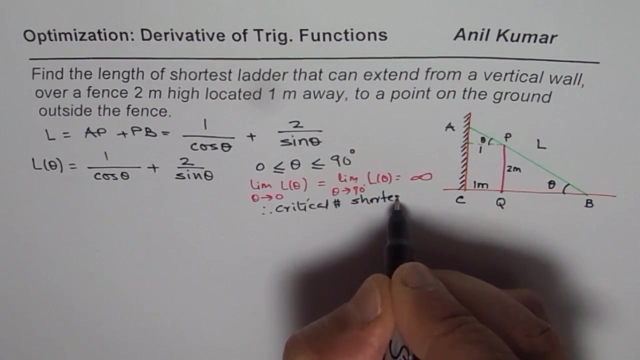 so that is also infinity right. So what we observe here is that the limit as theta approaches 0 for L theta is actually equals to the limit as theta approaches 90 degrees for L theta, and both are approaching infinity right. So that is how we can say that our critical number is going to be of shortest length. So 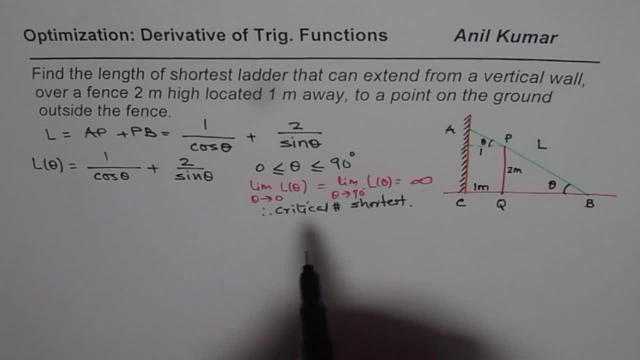 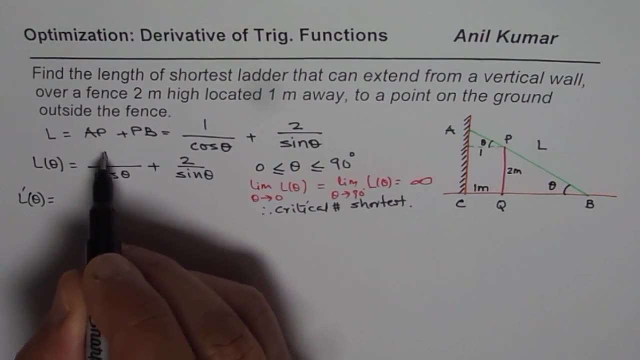 this is very important. Now to find the critical number, let us find the derivative. So what is the derivative Derivative of length with respect to angle theta 1 over cos theta? So what we can do is we can apply the quotient rule. So cos square theta 1 derivative is 0, so we will. 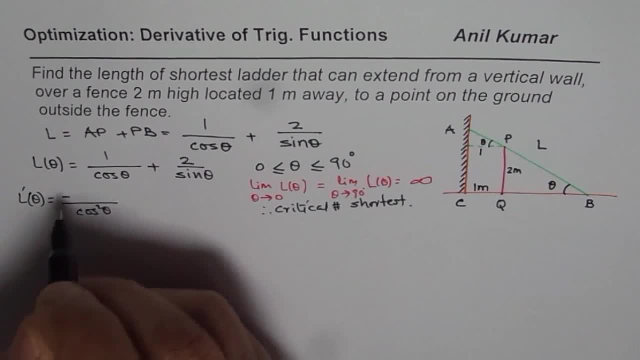 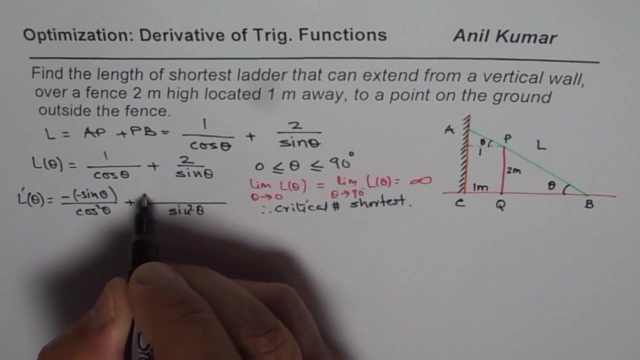 have 0 minus 1 times derivative of cos theta, which is minus sine theta. Let me write minus sine theta. So that is the first term. And for the second term, derivative of denominator is sine square theta 2 derivative is 0, so we get 0 minus 2 times derivative of sine. 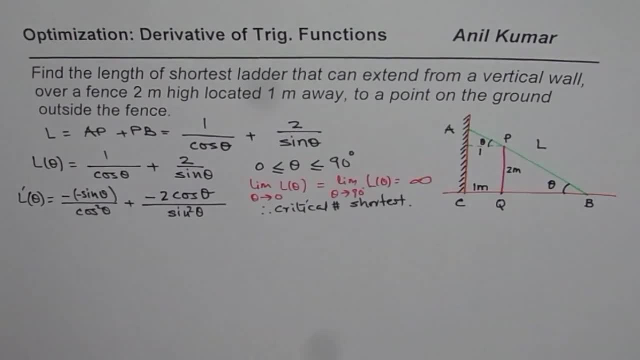 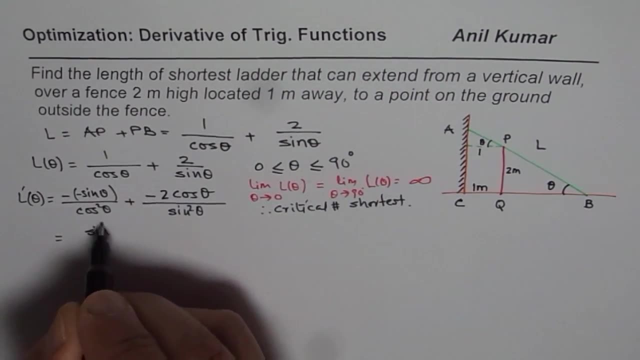 theta which is cos theta, So that becomes the derivative. Let us take the common denominator and simplify. So that gets multiplied here, So we get sine cubed theta, And on this side it is minus 2 cos cubed theta divided by sine square theta, cos square theta. Now for critical. 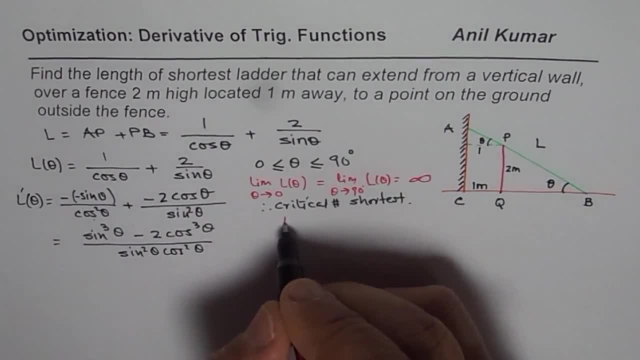 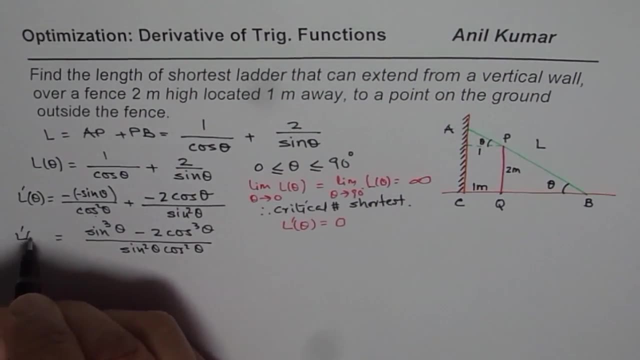 number, the derivative should be 0. So for critical number, derivative should be 0. So we can equate this to 0.. So that is our derivative. Let us equate to 0 and find the critical number. So that was it. 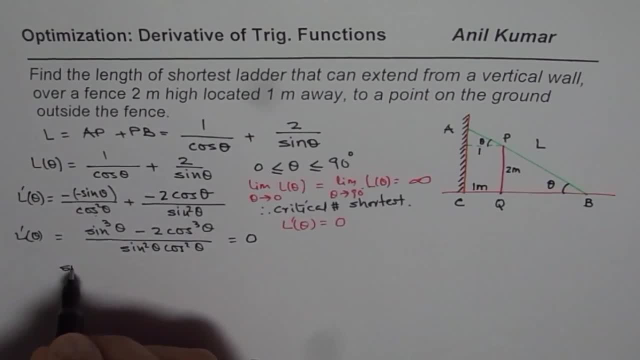 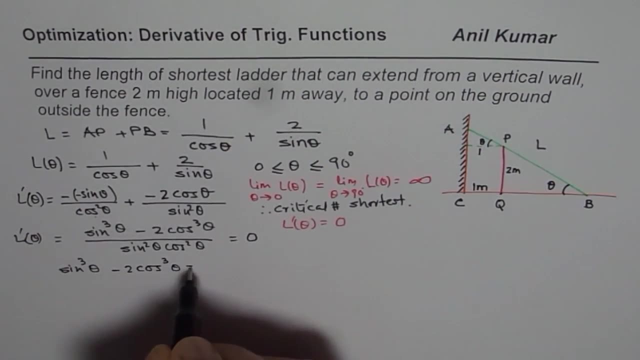 really means that the numerator is 0, that is to say that sine cube theta minus 2 cos cube theta equals to 0. so that means sine cube theta equals to 2 cos cube theta. or we can say: sine cube theta divided by cos cube theta equals to 2, and that is tan right which. 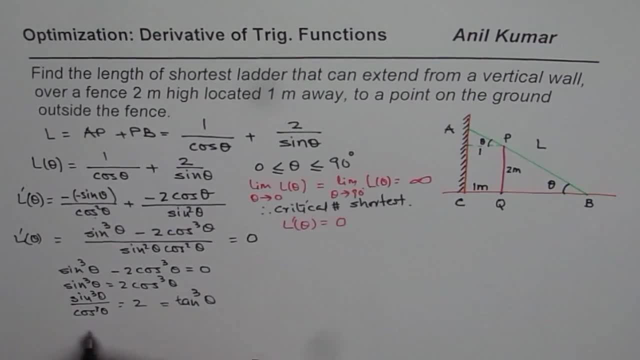 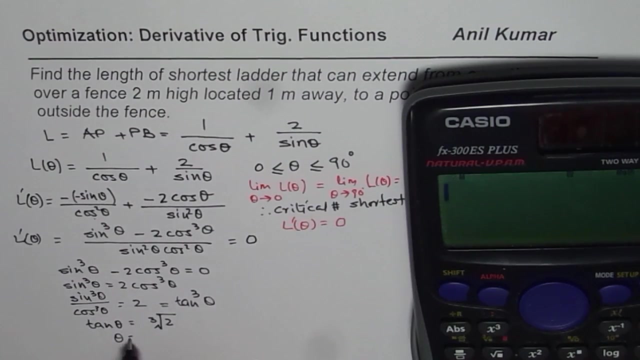 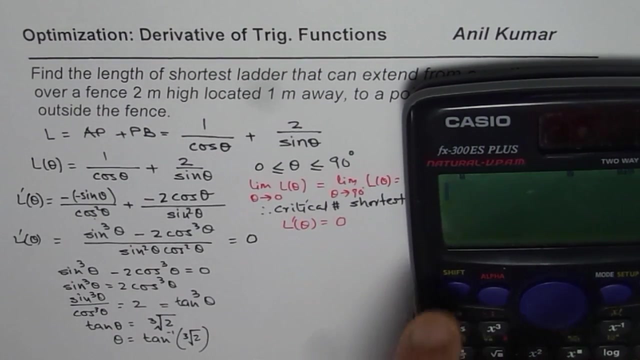 is tan cube theta right or tan theta equals to cube root of 2? we can use the calculator and find theta where. so we can say from here: theta equals to tan inverse of cube root of 2, right, so shift. tan inverse cube root is 0.. 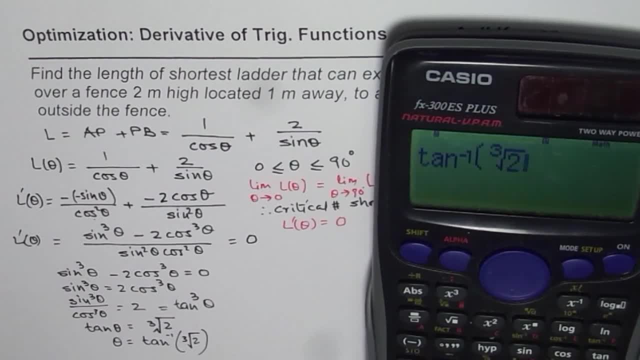 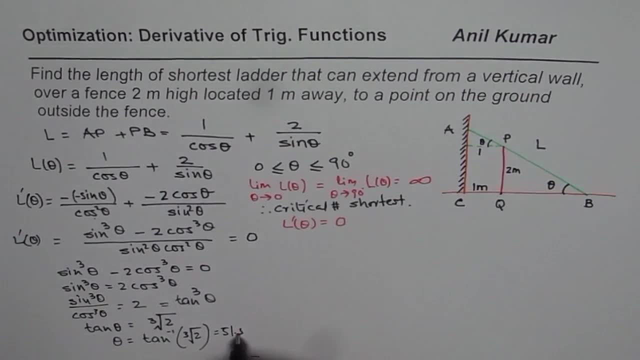 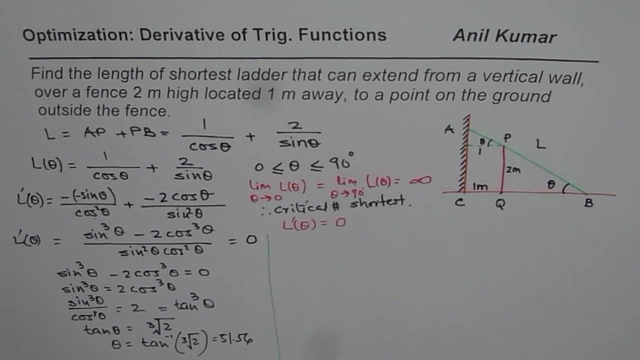 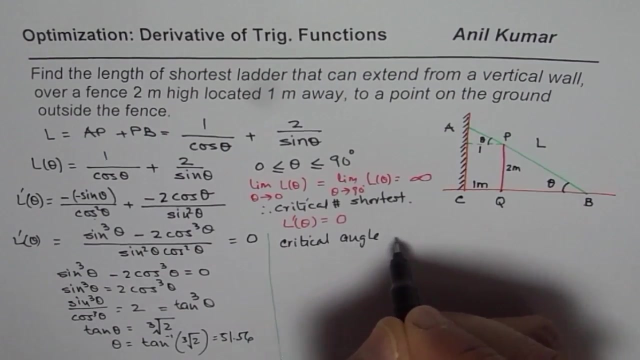 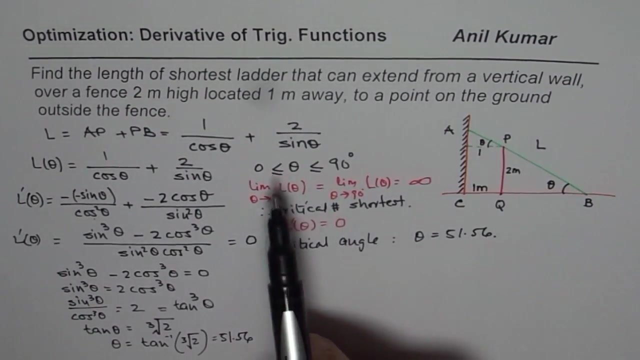 Here, cube root of 2 and bracket close equals to 51.56. so we get angle: theta equals to 51.56. so what we get here is the critical angle. so we say critical angle for us is theta equals to 51.56, since we know that because of the boundary conditions we are getting length infinitely. 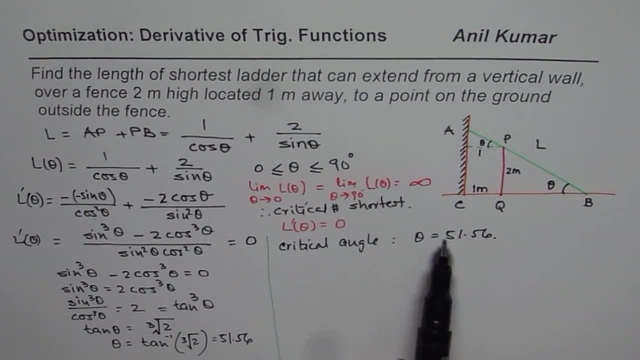 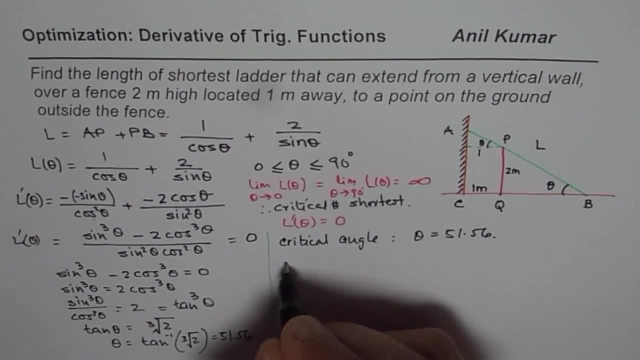 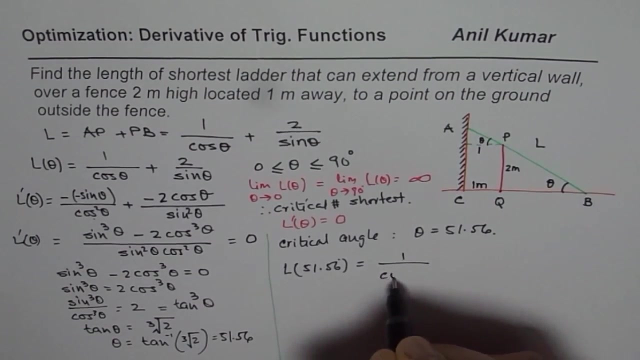 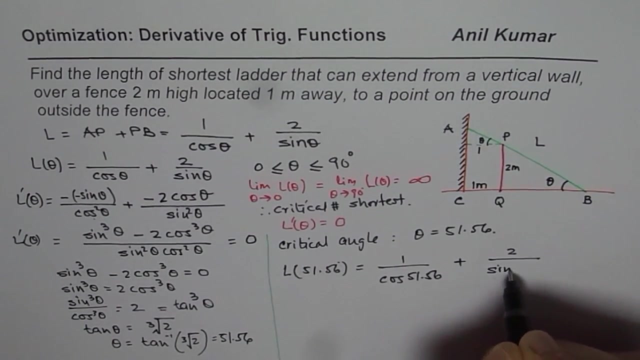 large critical number will give us a shorter length, right? so that is the angle at which we'll get the shortest length. so let's now find the length. so what is the length? for 51.56 degrees, that is equals to 1 over cos of 51.56 plus 2 over sine of 51.56 degrees. 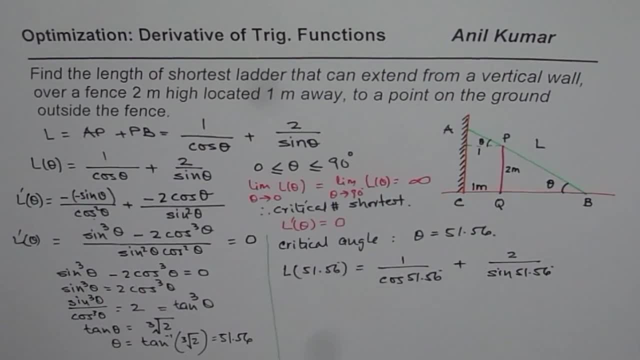 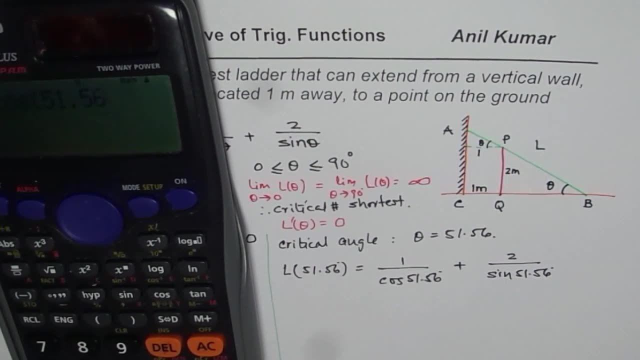 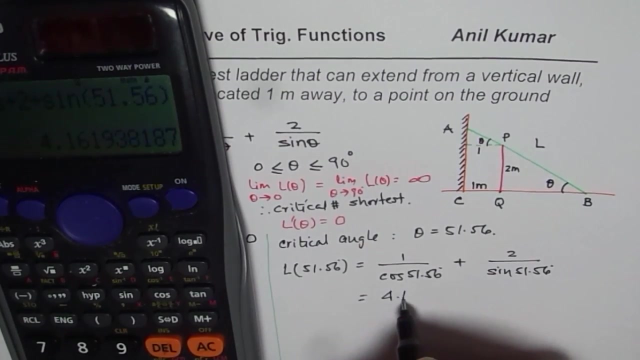 1.56 degrees, right? Let's calculate this. So we have: 1 divided by cosine 51.56 plus 2 divided by sine 51.56 equals 2.. So that gives us approximately 4.16, right? So the? 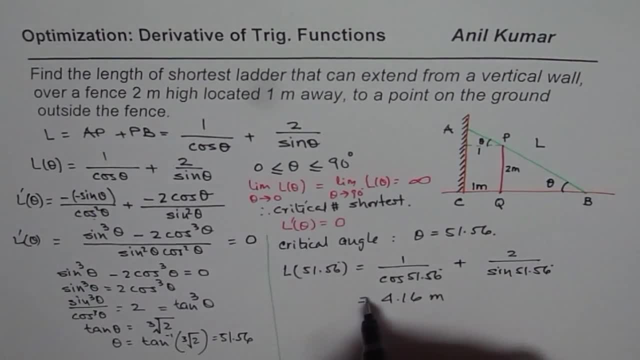 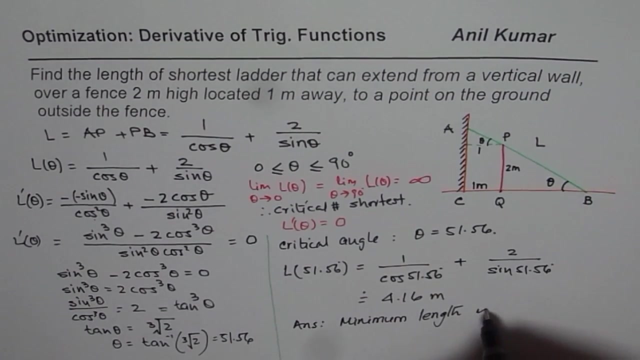 dimension is 4.16 in meters, So that is the minimum length of the ladder, right? So from here we get our answer and that is, minimum length is 4.16 meters. I hope the steps are absolutely clear. So very first step should always be, depending on the situation, sketch: 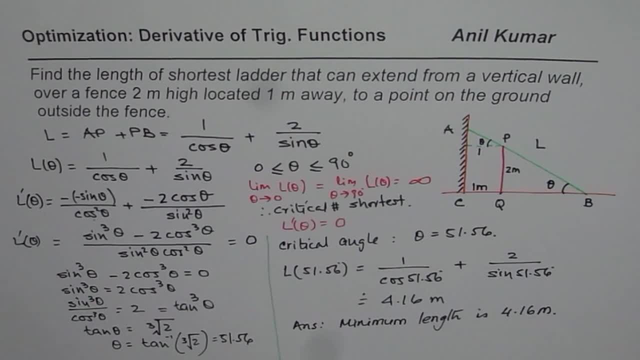 a neat diagram. Define your variables. Now we used trigonometry to solve this question and wrote: we have used trigonometry to solve this question. wrote angle theta as the angle which ladder makes with the horizontal or the ground. Now writing L in terms of 1 over cos theta plus. 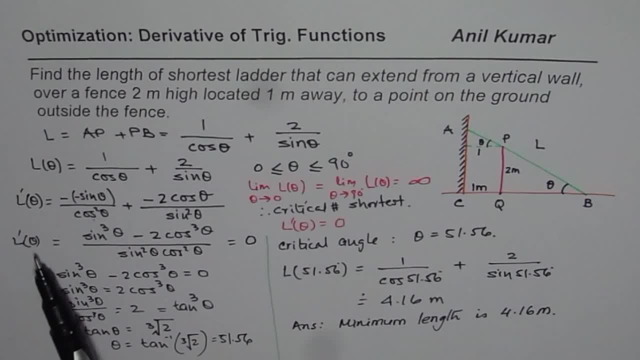 2 over sine theta helps us to find the derivative With respect to the angle theta, and the critical number here represents the shortest side, since the boundary conditions will give us infinitely large value. This is a very important concept. Once you find the critical number, substitute and find the length of the ladder. Now this: 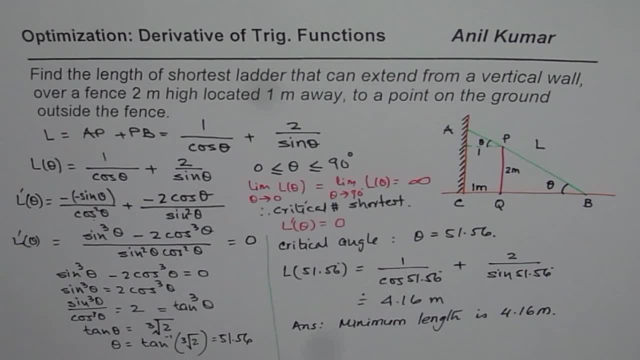 question is extremely important. We have similar questions in many test papers. I'd like you to understand the concept and then try out some questions from your book. I hope that helps. Thank you And all the best.